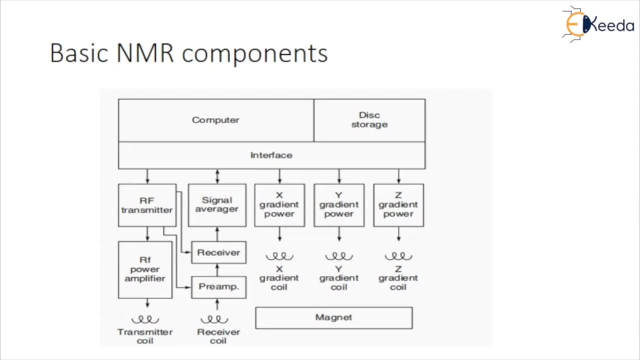 The pulses are amplified to the level of C1.. to the levels varying from 100 watt to several kilowatt, depending on the imaging method, and are fed to the transmitter coil. The higher power levels are necessary for the large sample volumes encountered in the whole body experiments. The RF coils can be either a single coil serving 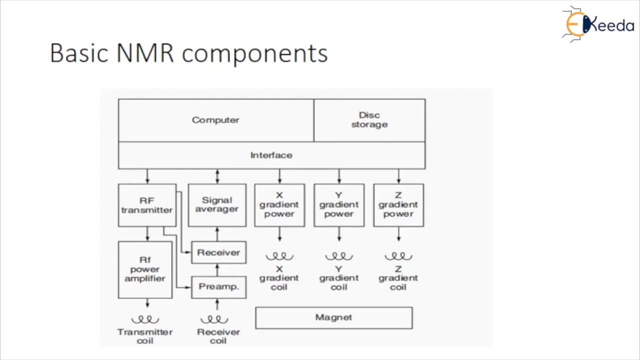 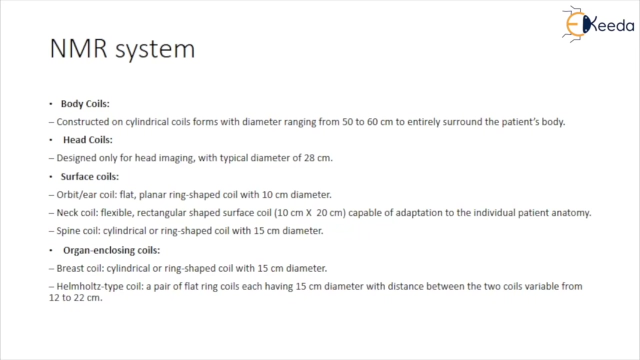 both transmitter and receiver or two separate coils that are electrically orthogonal. Detection System. The function of the detection system receiver is to detect the nuclear magnetization and generate an output signal for processing by the computer. NMR system has the following available coils: Body coils constructed a cylindrical coil forms with a diameter ranging from 50 to 60. 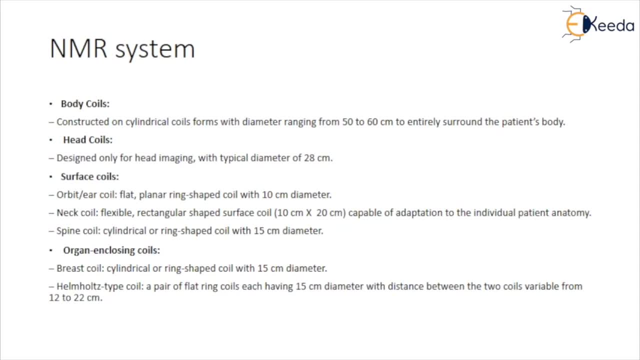 cm to entirely surround the patient body. Head coils designed only for head imaging, with typical diameter of 28 cm Surface coil. Orbit or ear coil: Flat planar ring shaped coil with 10 cm diameter Neck coil- Flexible, rectangular shaped surface coil capable of adaptation to the individual parent anatomy. 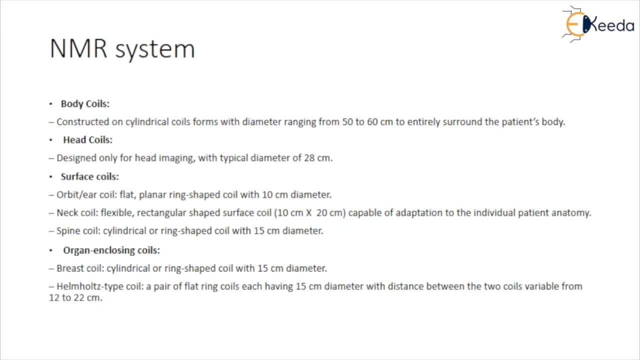 and spine coil- Cylindrical or ring shaped coil, with 15 cm diameter. Organ enclosing coils. Breast coil- Cylindrical or ring shaped coil- with 15 cm diameter. Stiff type coil. A pair of flat ring coils, each having 15 cm diameter, with distance between: 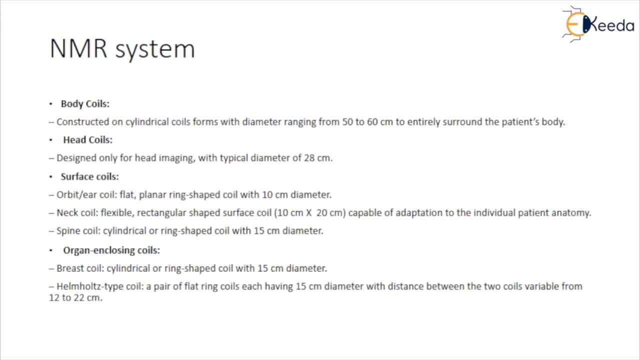 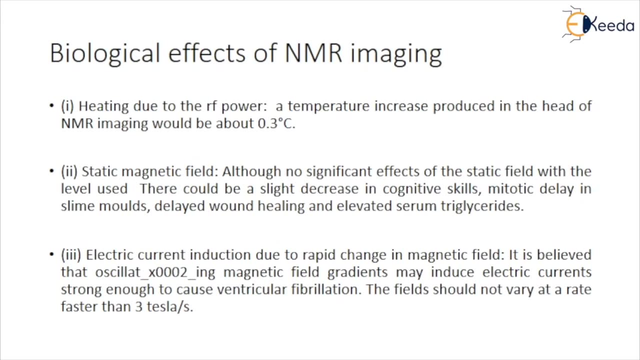 the two coils, variable from 12 to 22 cm. Biological effects of NMR imaging. Hitting due to the RF power that reports, the temperature increase produced in the head of the NMR imaging would be about 0.3°C. This does not seem likely to pose a problem, But static magnetic field, although no significant, 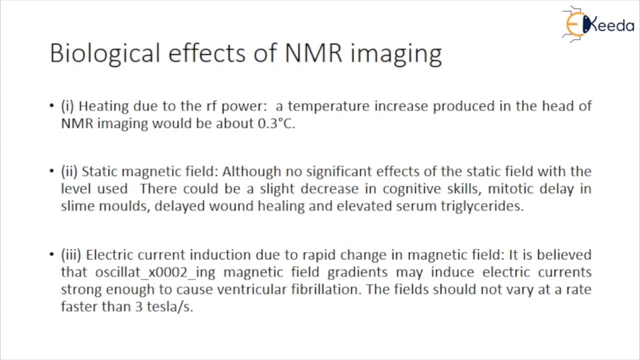 effects of the static field. with the level used in NMR that the possible side effects of electro-magnet fields, there could be a slight decrease in the cognitive skills, Mito-tick delay in the sling modules, delayed wound healing and elevated serum triglycerides. 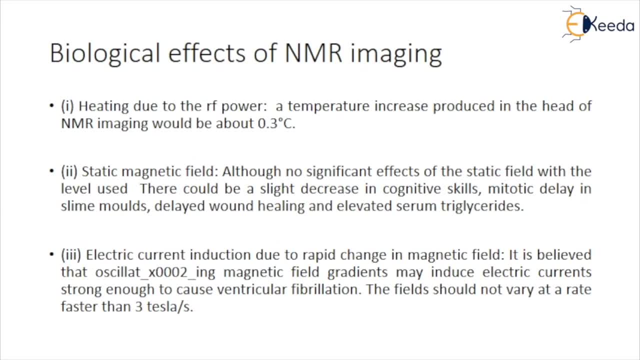 Electric current induction. Due to the rapid change in the magnetic field, it is believed that osc magnetic field gradient may be depleted even after 5-6 years. magnetic field gradients may be induced electric currents strong enough to cause ventricular fibrillation. No damage due to the NMR from exposure have been reported, but it is still. 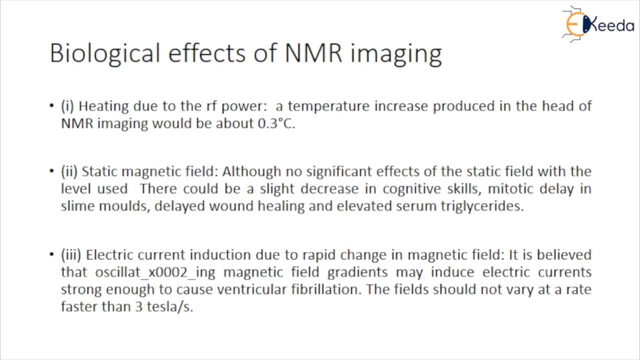 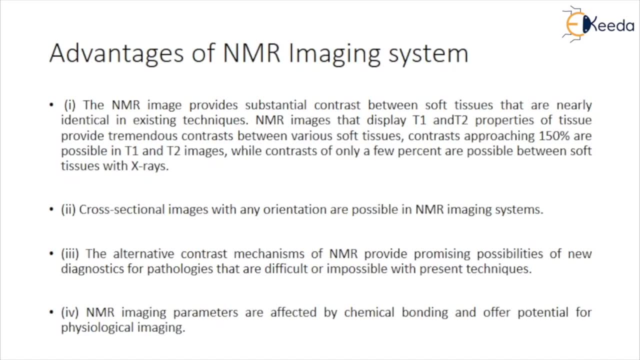 suggested that the field should not vary at the rate faster than 3 Tesla per second. Advantages of NMR Imaging. The NMR images provide substantial contrast between soft tissues that are nearly identical in existing NMR images that display T1 and T2 properties of tissue. provide tremendous contrast between various soft tissues. 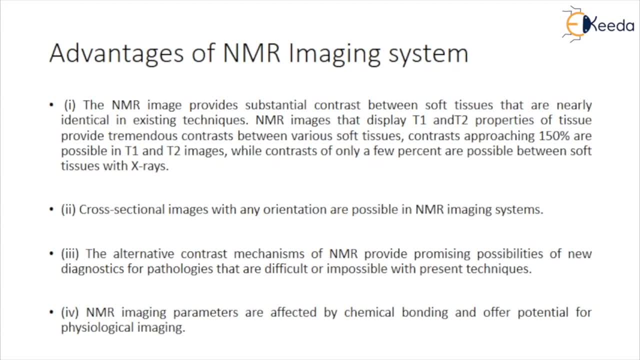 Contrasts approaching 150% are possible in T1 and T2 images, while contrasts of only few percent are possible between soft tissues with X-rays. Cross-sectional images with any orientation are possible in NMR imaging systems. The alternative contrast mechanism of NMR provide promising 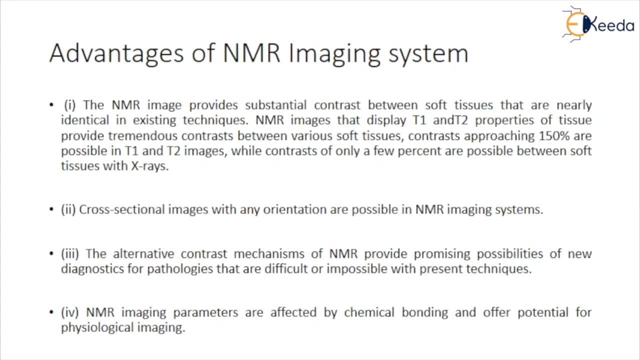 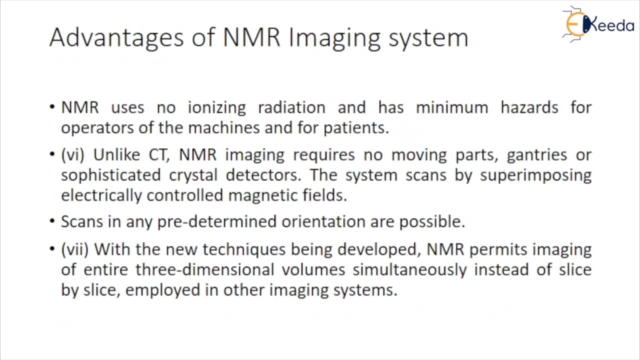 possibilities of new diagnostics for pathologies that are difficult. NMR imaging parameters are affected by chemical bonding and offer potential for physiological impact. NMR uses no ionizing radiation and has minimum hazard for operators of the machine and the patients. also, Unlike CT, NMR imaging requires no moving parts, gantries or sophisticated 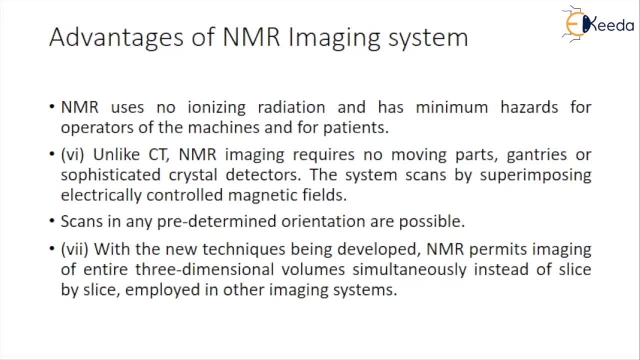 crystal detectors. The system scans by superimposing electrically controlled magnetic fields. Scans in any region of the body are possible. NMR imaging parameters are affected by chemical bonding and has minimum hazard for operators of the machine and the patients. also, Contrasts approaching 150% are possible in NMR imaging systems. 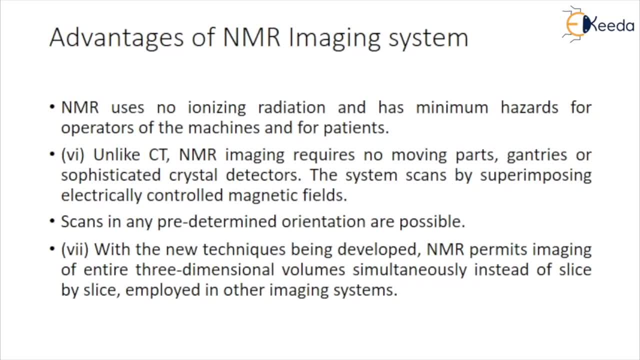 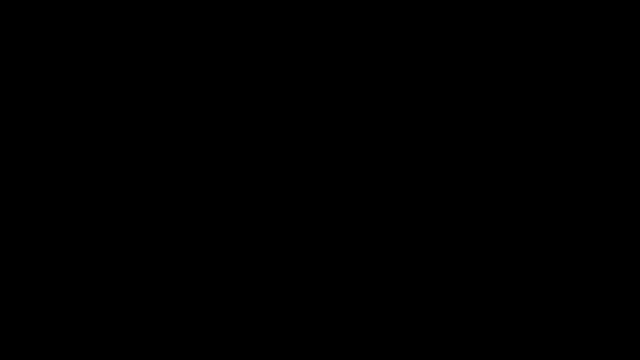 With the new techniques being developed. NMR permits imaging of entire three-dimensional volumes simultaneously, instead of slides by slides employed in other imaging systems. you.